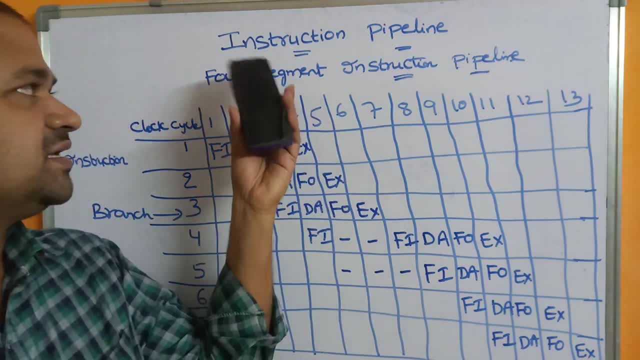 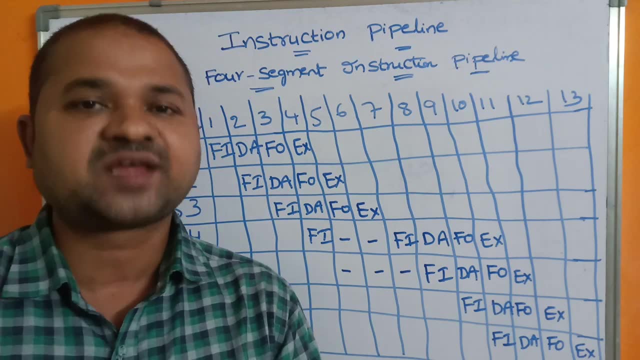 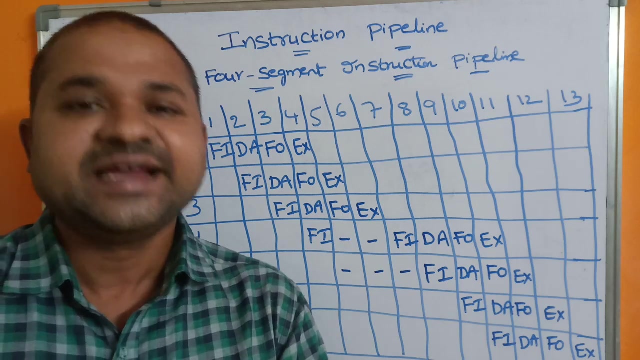 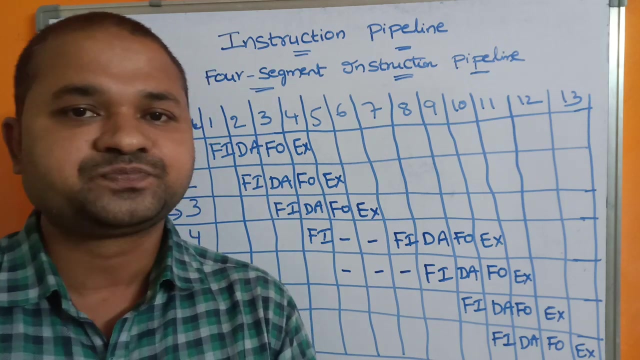 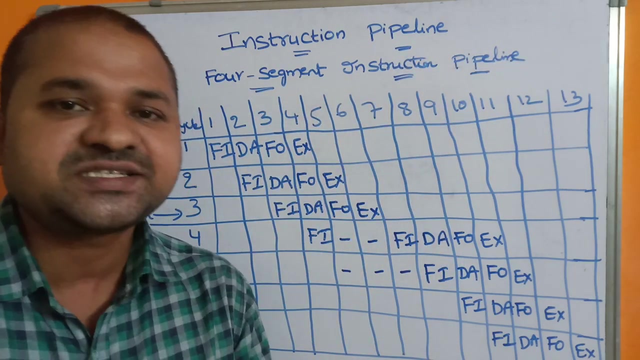 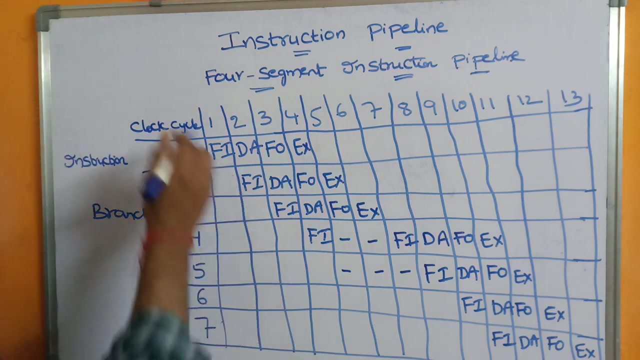 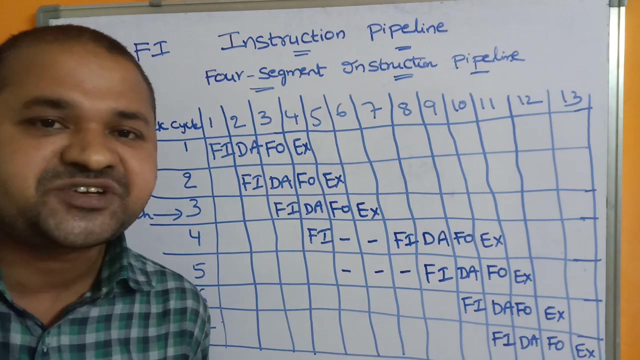 In this video we are going to discuss about instruction pipeline. Pipelining is mainly useful in order to enhance the performance of a computer. We know that program means a collection of instructions. Here we can execute multiple instructions concurrently. Here let us take the example of a four-segment instruction pipeline. So that means we can execute the corresponding instruction by using four segments. The first segment is FI. FI stands for fetching of instruction from the memory. 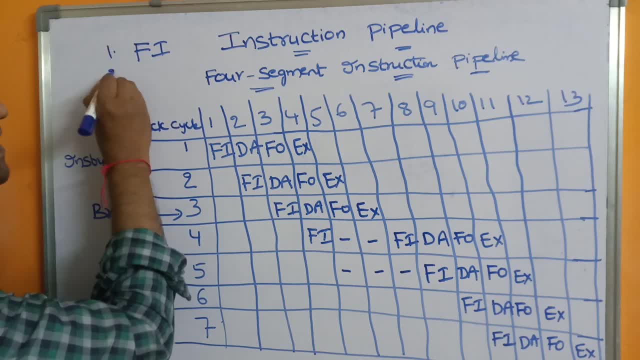 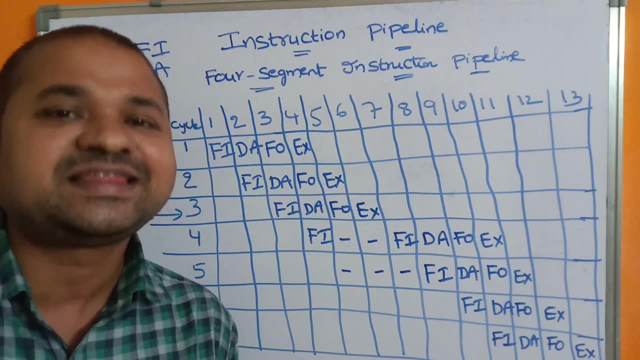 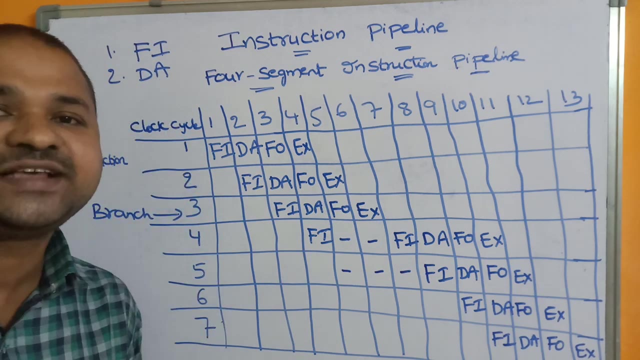 And the second segment is DA. DA stands for decode instruction from the memory, DA stands for decoding the instruction and finding the effective address. So D stands for decoding the instruction, A stands for effective address, A stands for address and calculating the effective address. 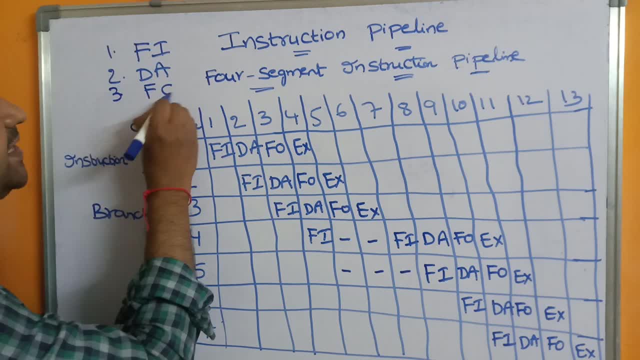 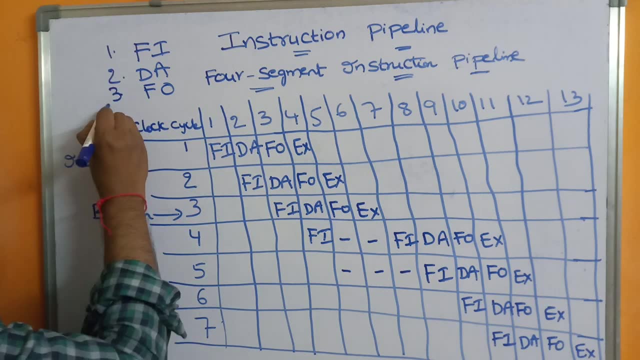 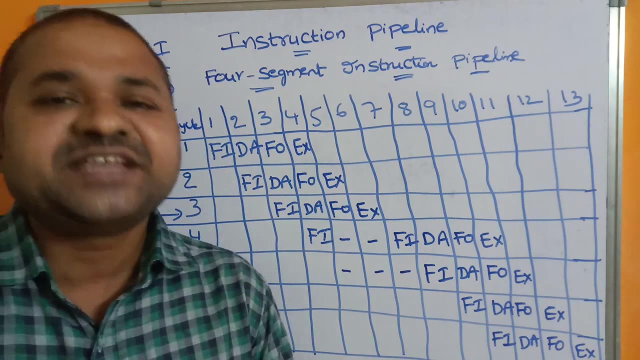 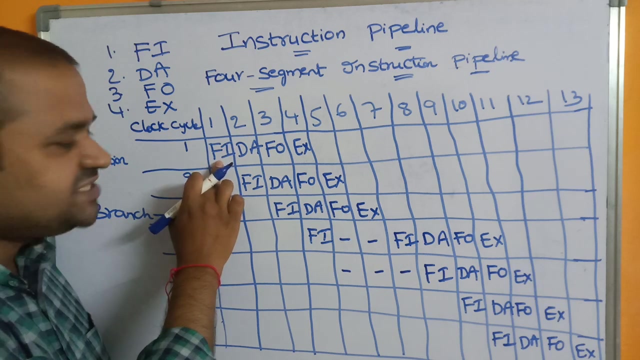 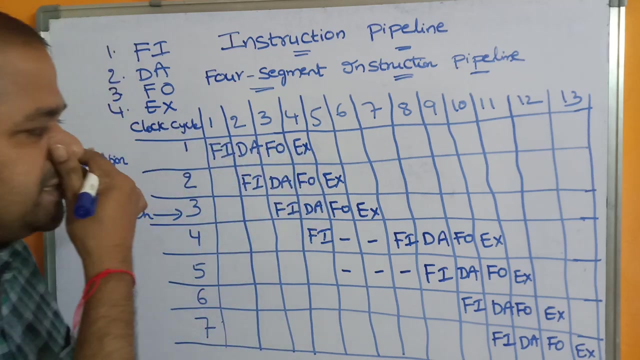 And the third segment is FO- FO stands for fetching operand. And the fourth segment is EX- EX stands for executing the instruction. So each instruction is executed by using these four segments: FI, fetching of instruction, DA- decoding the instruction and finding the effective address. Fetching the operand and executing the instruction. 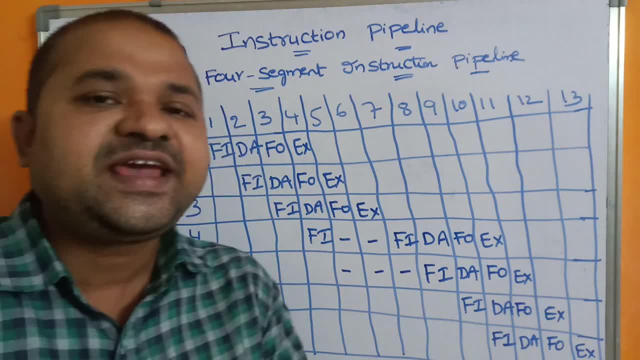 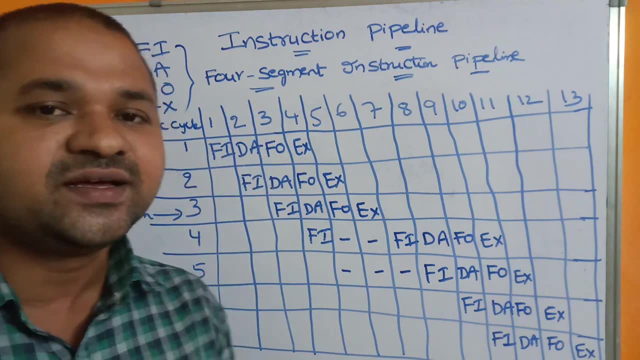 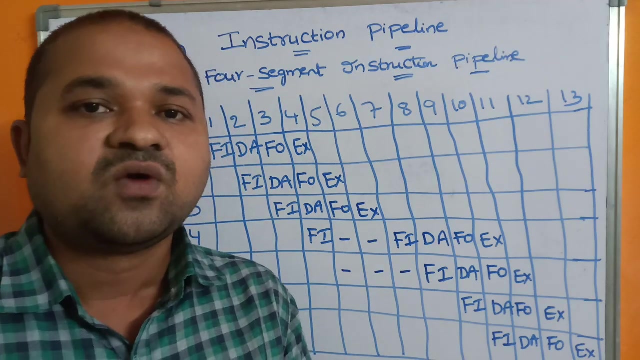 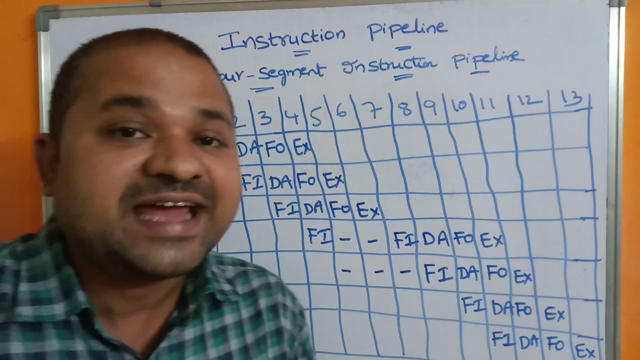 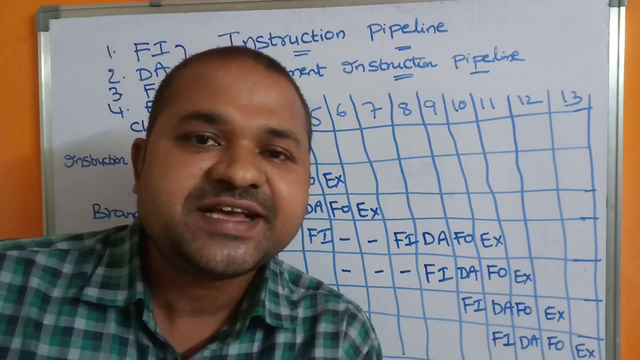 Here we can execute multiple instructions concurrently simultaneously by executing the corresponding instructions. So that means, while fetching first instruction, we can execute the second instruction, second segment, And we can execute third instruction, third segment, We can execute fourth instruction, fourth segment. 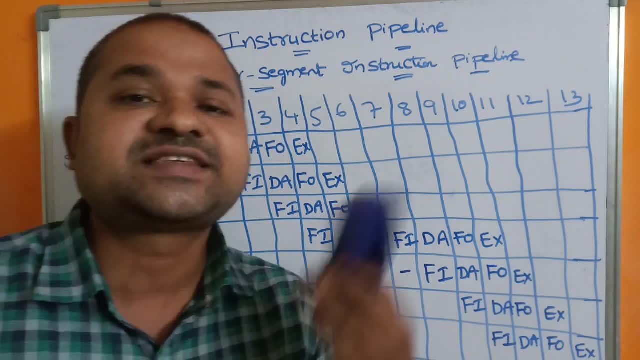 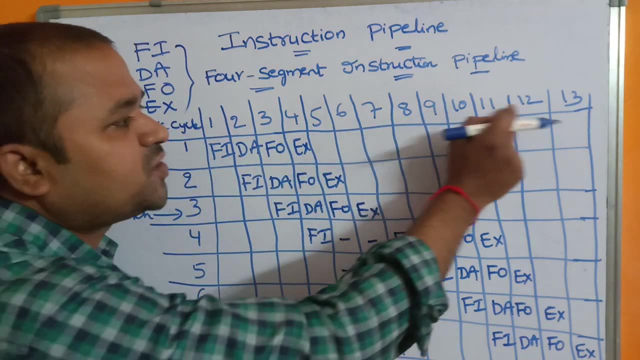 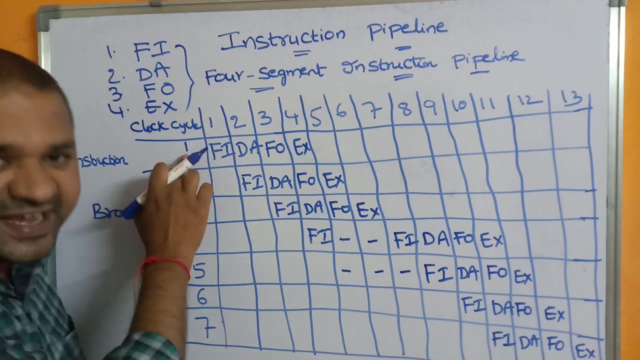 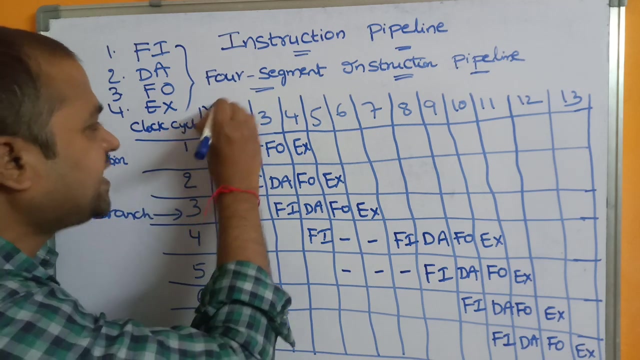 So we can do all these four activities simultaneously here. So let us see this diagram. So here this is nothing but a collection clock cycle. So totally we have 13 clock cycles are there and this y-axis represents instructions. So totally there are 7 instructions are present. So during first clock cycle 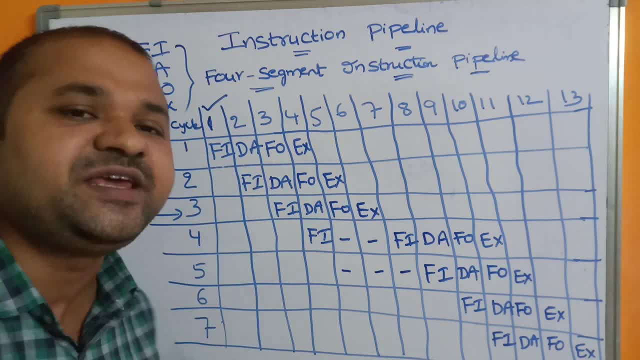 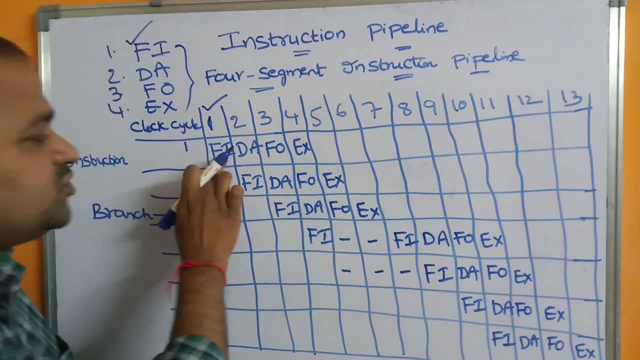 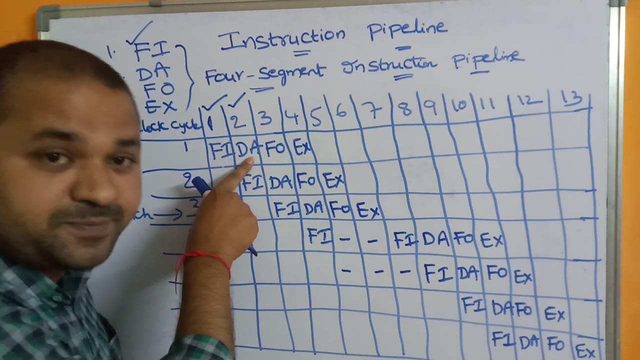 the first instruction, first segment, is being executed. So what is the first segment of every instruction? So fetching the instruction, So that is executed. Next, during second clock cycle, the first instruction segmented to as well as the second instruction first. 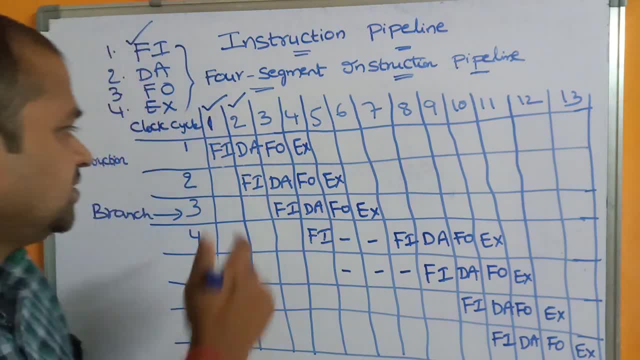 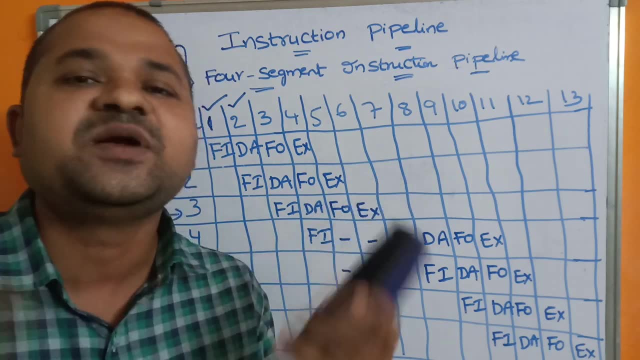 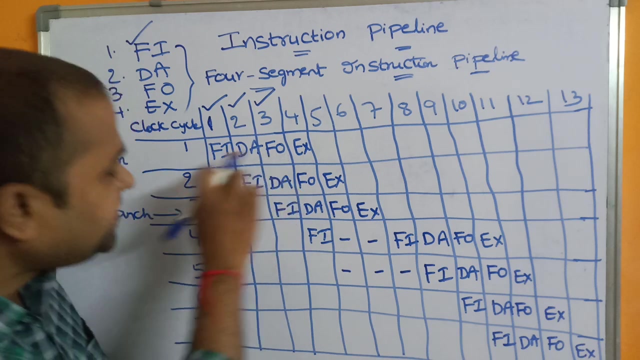 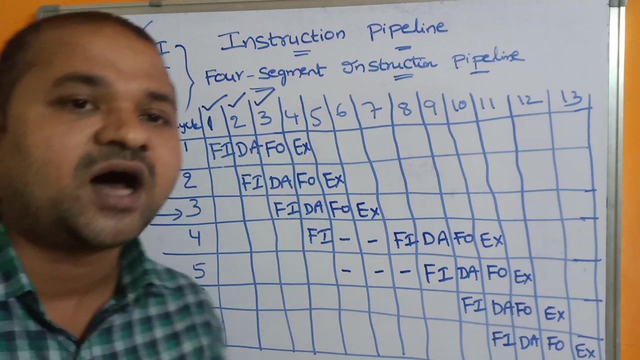 segment is being executed. So that is the advantage of pipelining: We can execute multiple instructions, multiple segments, simultaneously, And during the third clock cycle, the first instruction- third segment, second instruction- second segment, as well, As well as third instruction- first segment, are being executed. Now let us see the fourth. 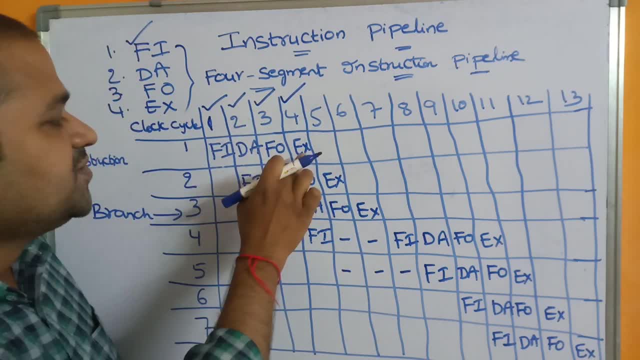 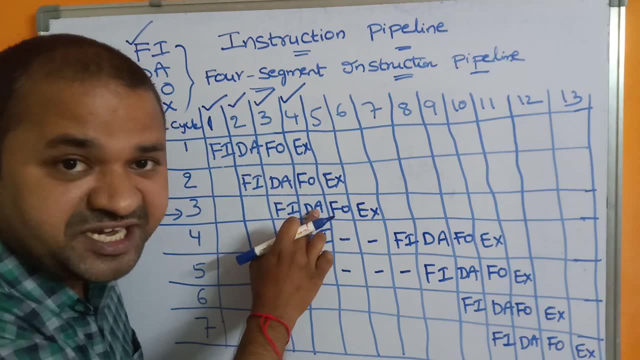 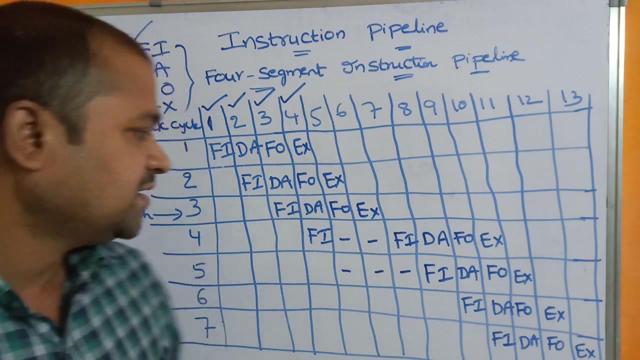 clock cycle. So during fourth clock cycle, first instruction, segment 4, second instruction, segment 3, third instruction, second segment, as well as fourth instruction. first segment is being executed Here. let us assume that now we are at the fourth clock cycle. So 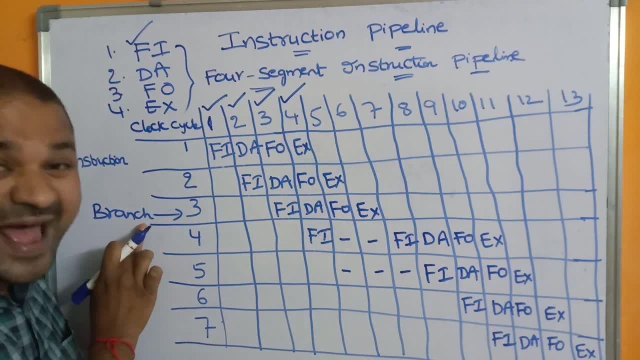 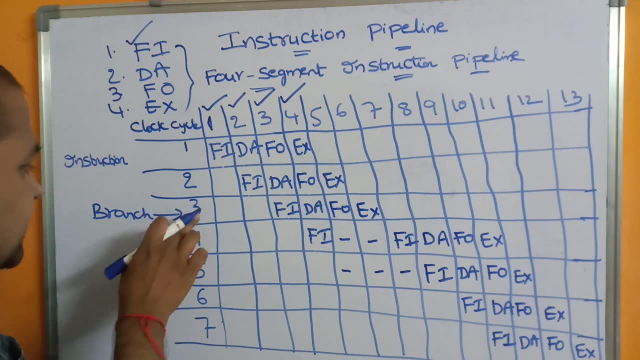 let us assume that third instruction is a branch instruction. So during the decoding, the, during this phase, we came to know that this third instruction is a branch instruction. So first let us see what is a branch instruction. So let us assume that we are here at 100 address. 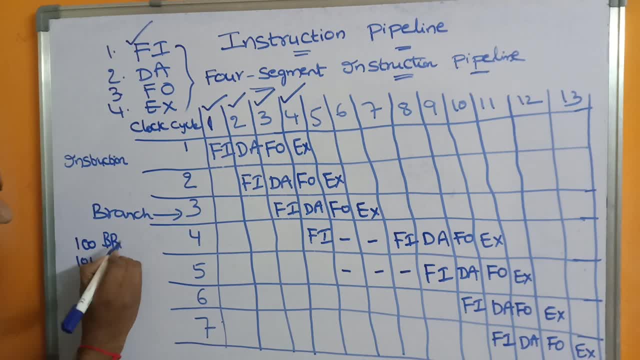 Let the next address is 101.. So we are executing branch instruction. Let the address here is 301.. Suppose if the condition is satisfied, then program counter will become 301. So that means the instruction at the address 301 will be executed. Suppose if this condition is. 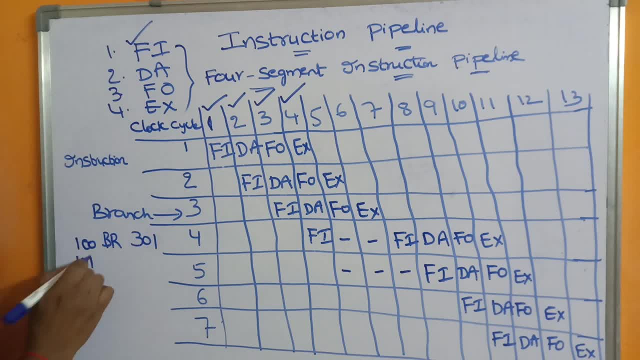 false. if BR condition is false, then the next instruction will be executed. So what is the next instruction? So the instruction at address 101 will be executed. So here, what is the third instruction? here The third instruction is the branch instruction, So we cannot fetch any other instruction. 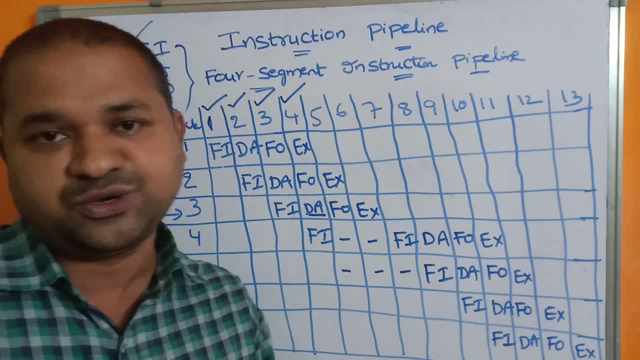 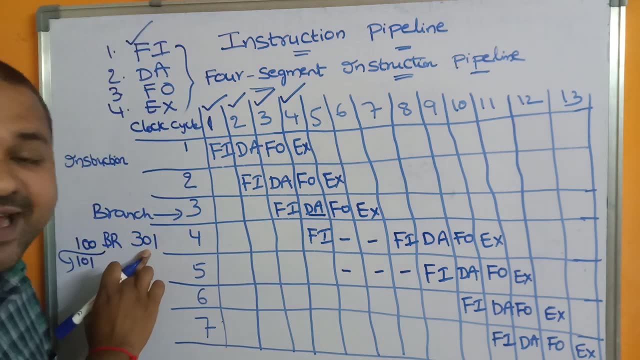 until the branch instruction is successfully executed. Why? because if the branch instruction condition is true, then we have to load a new instruction from the memory. We should not suppose if this condition is true then we should not fetch the next instruction. We have to fetch the instruction at the address 301.. So we 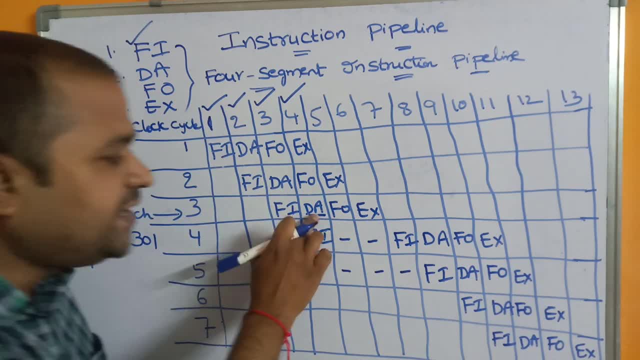 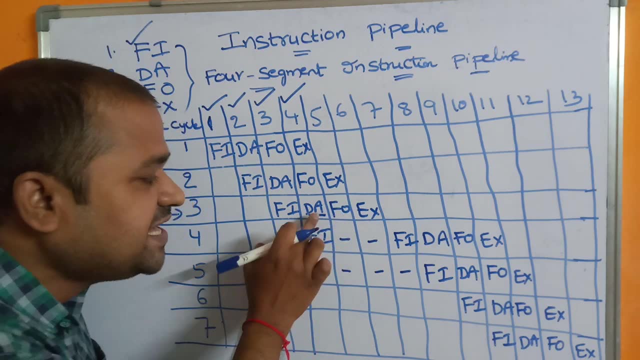 should not fetch the next instruction before we can run our safety. This is the second instruction, after which will see branch instruction control. So Then after We are running section joy. So here the point is, we cannot fetches any instruction from the memory until this instruction is successfully executed. So that is why let us see the 5th clock cycle. 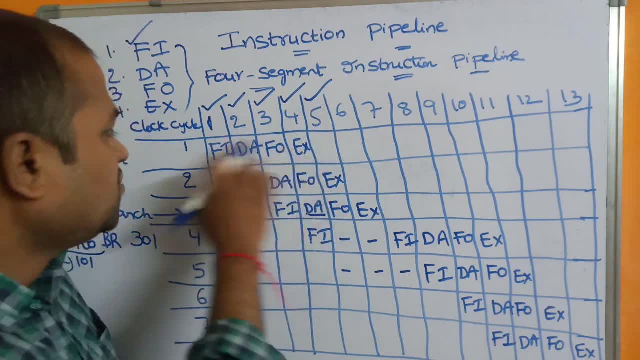 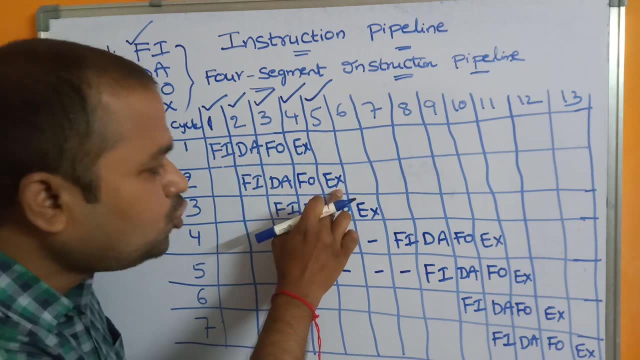 So during the 4th clock cycle, this first instruction is successfully executed. So during the 5th clock cycle, what we are doing here? Instruction 2, segment 4, as well as instruction 3, segment 3 are being executed. 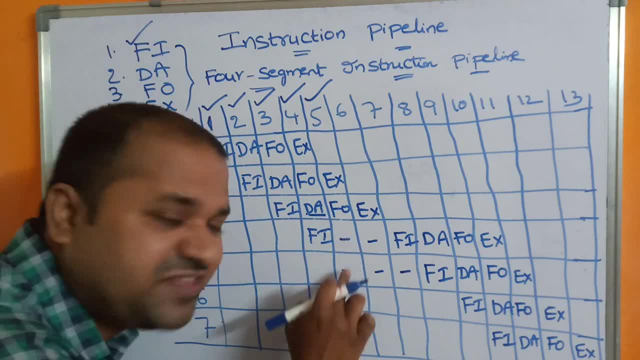 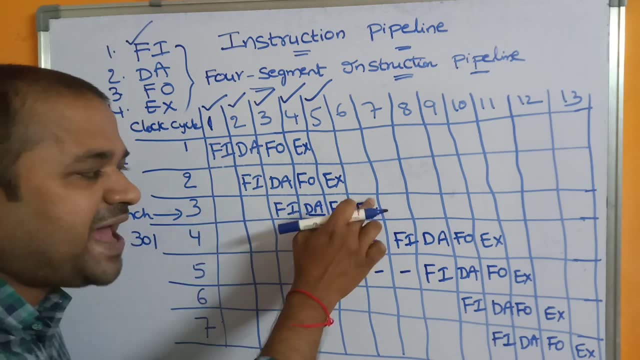 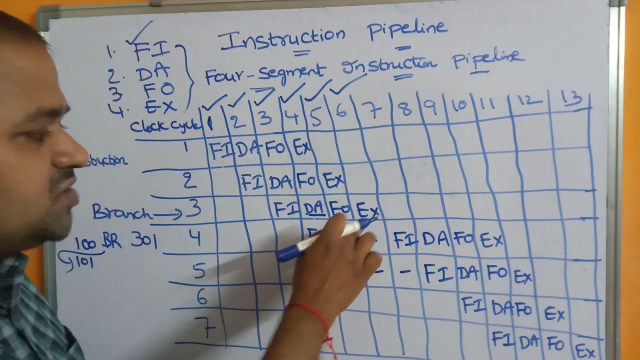 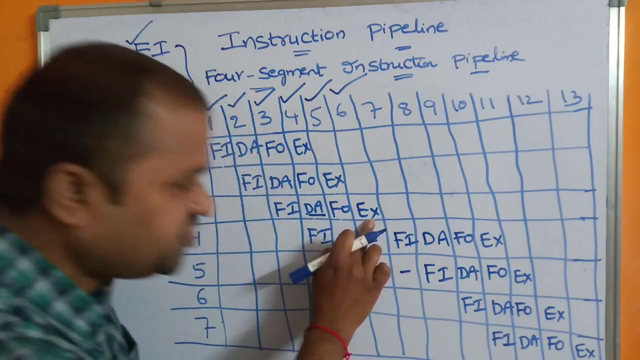 But we are not fetching any other instruction here. Why? Because we have to fetch the next instruction only after executing the branch instruction, Only after executing the branch instruction. So, after executing the 3rd instruction, let us observe the 6th clock cycle. So, during 6th clock cycle, we have successfully executed the 3rd instruction, that is, branch instruction. 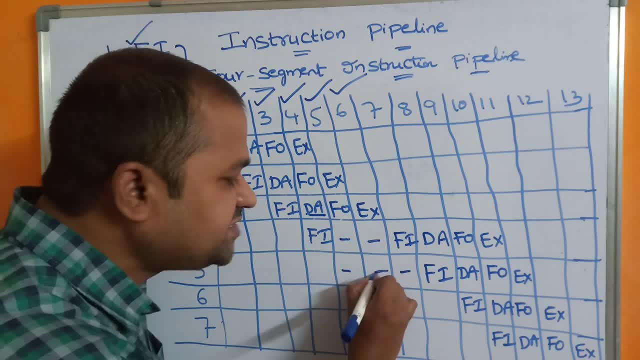 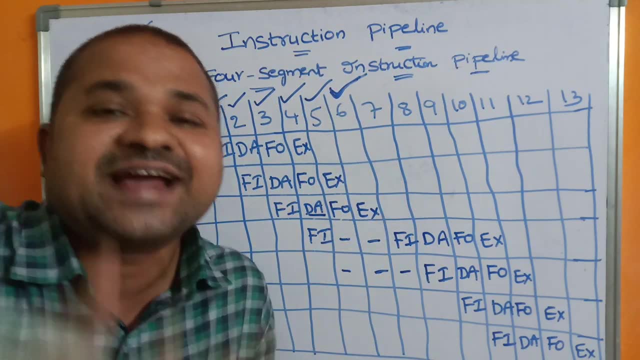 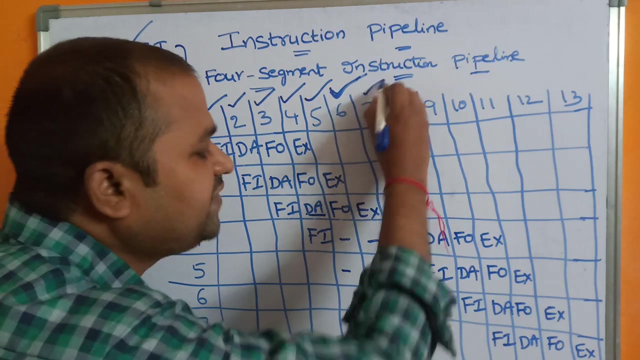 So next here: no instruction is fetched here. no instruction is fetched here. So after the end of 6th clock cycle we came to know the next instruction address. So now that instruction is fetched from the memory. So during the 7th clock cycle we have fetched. 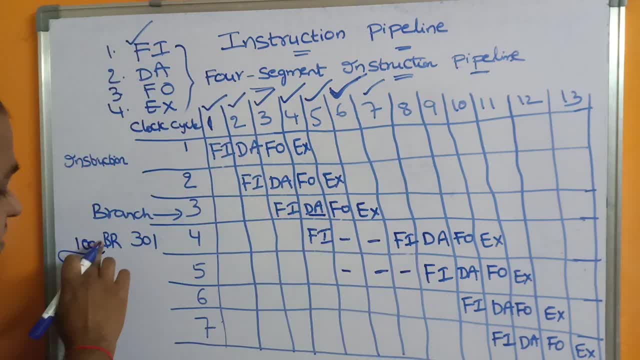 We have fetched the next instruction from the memory. Suppose if the condition is true, then 301 is the corresponding instruction address. Suppose if the condition is false, then what will happen? This 101 will be the address here. This 101 will be the address. 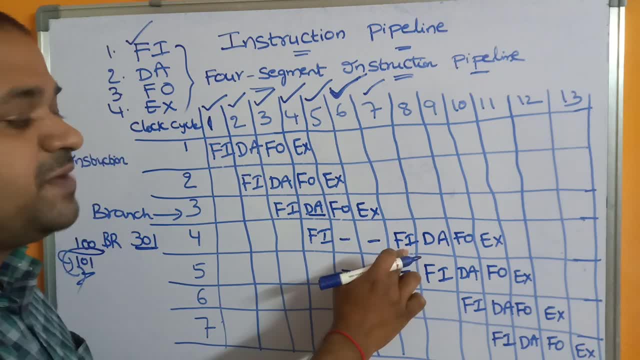 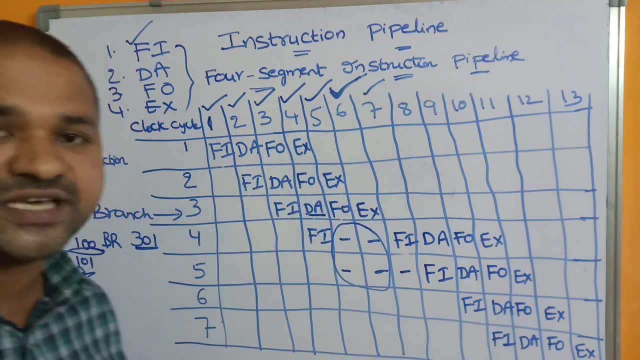 So during 7th clock cycle, instruction 4 is fetched from the memory, So here this is the problem here. So during this 6th clock cycle, as well as 7th clock cycle, we are not utilizing 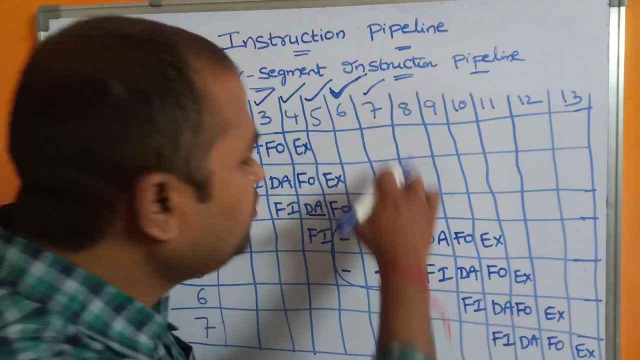 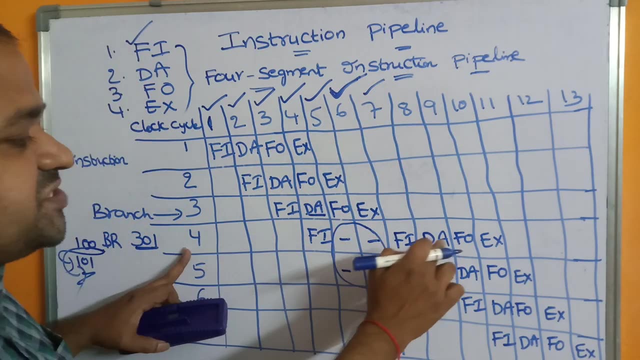 We are not using the pipeline in effect 2 manner. So during the 7th clock cycle, what is happening? We are fetching the 4th instruction. So during the 8th clock cycle, 4th instruction 2nd segment, as well as 5th instruction 1st segment is being executed. 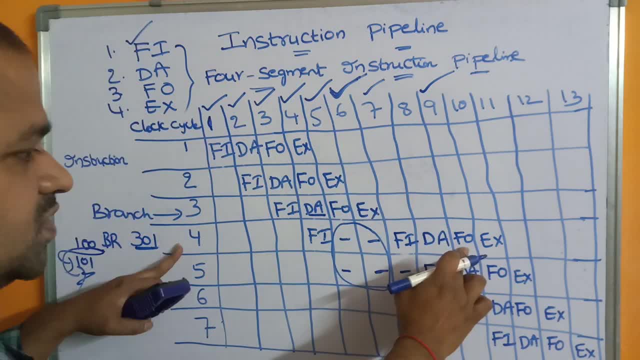 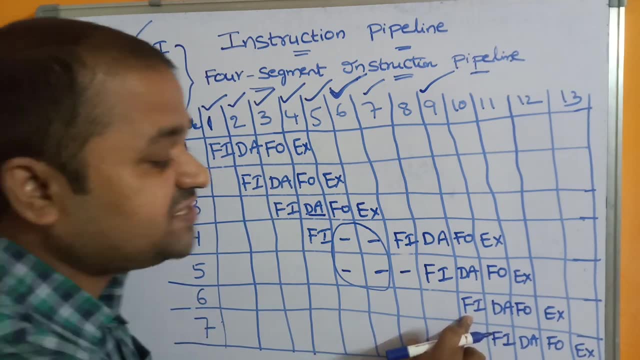 So during the 9th clock cycle, 4th instruction 3rd segment, 5th instruction, 2nd segment, as well as 6th instruction 1st segment will be executed. So likewise we are executing the instruction. 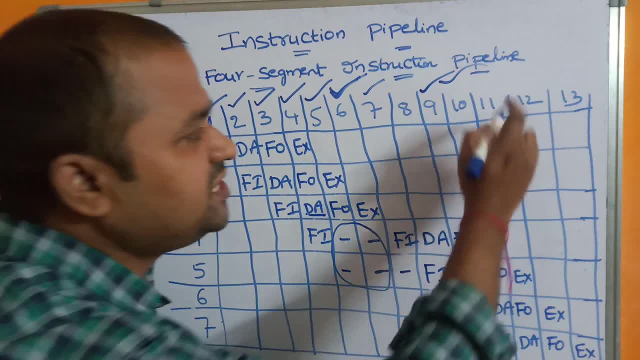 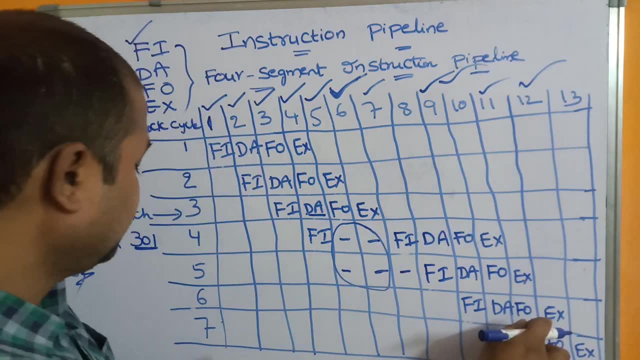 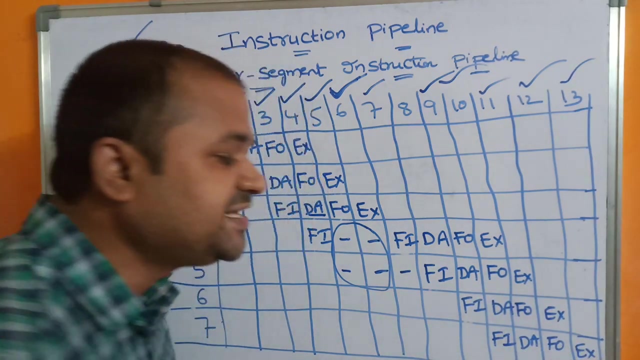 So during 10,, instruction 4 is successfully executed. During 11th clock cycle, instruction 5 is successfully executed. During 12th clock cycle, instruction 6 is successfully executed, as well as during 13th clock cycle, instruction 7 is successfully executed. 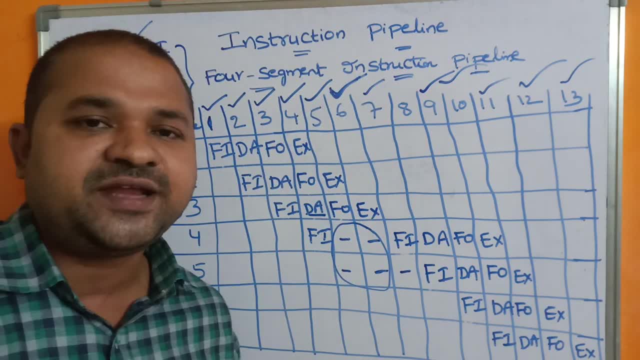 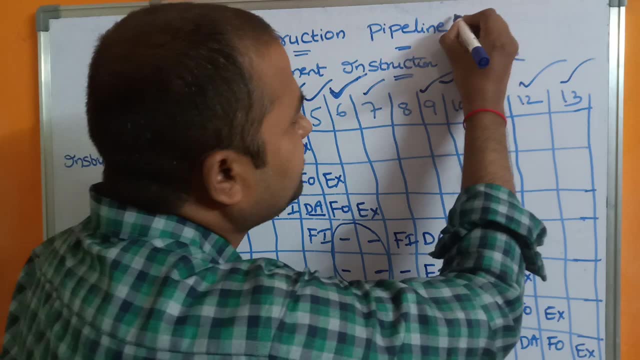 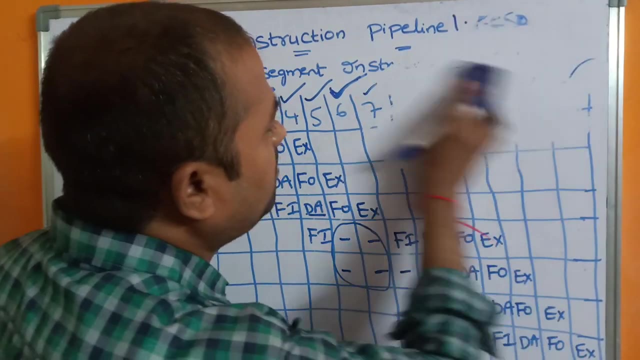 Here let us see the problem with the instruction pipeline. Instruction pipeline mainly suffers with 3 problems. So let us see those 3 problems now. The first problem is resource conflicts. So what is the first problem? The first problem is it suffers with 3 conflicts. 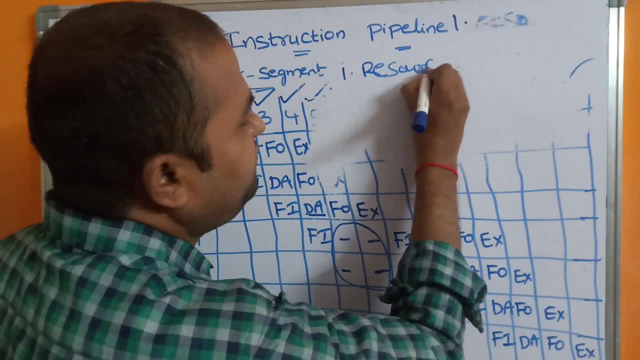 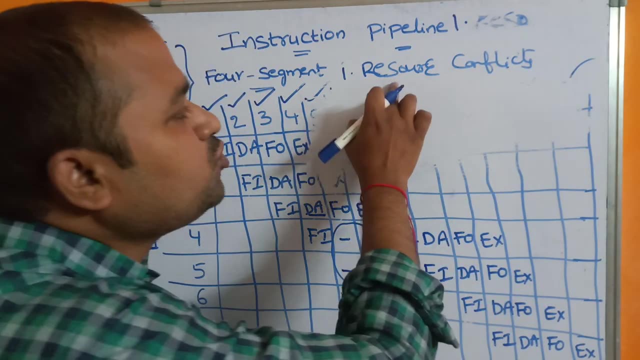 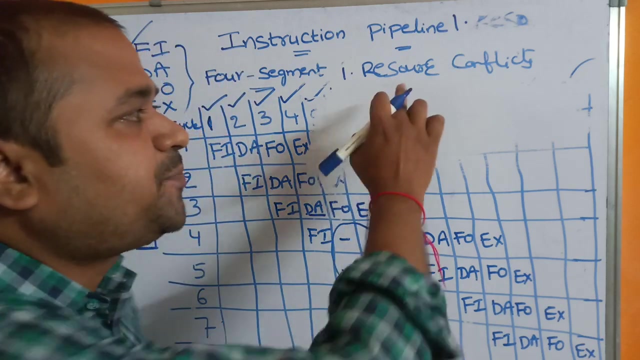 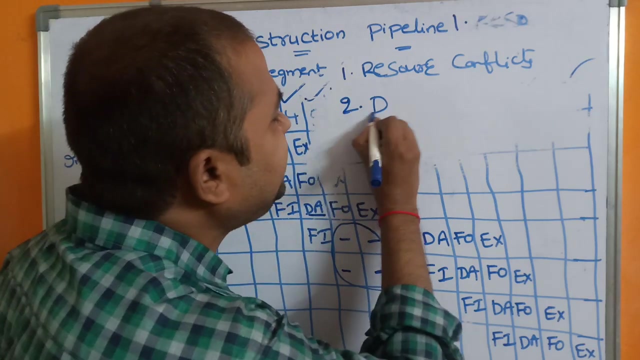 The first problem is resource conflicts. Resource conflicts means when multiple segments are trying to access the same resource simultaneously. then it leads to wrong results And that problem is called as resource conflicts- Resource conflicts. And the second problem is data dependency conflict. And the second problem is data dependency conflict. 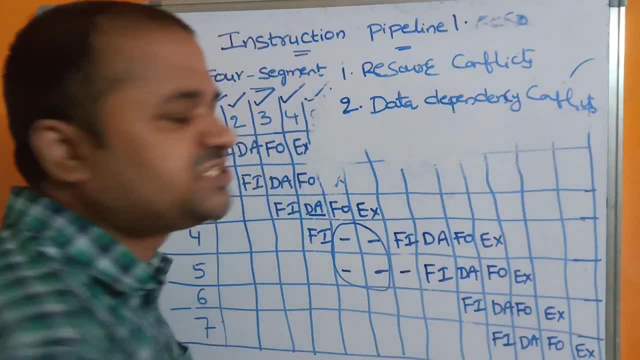 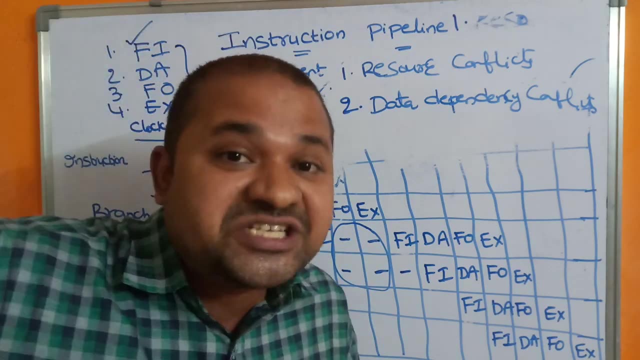 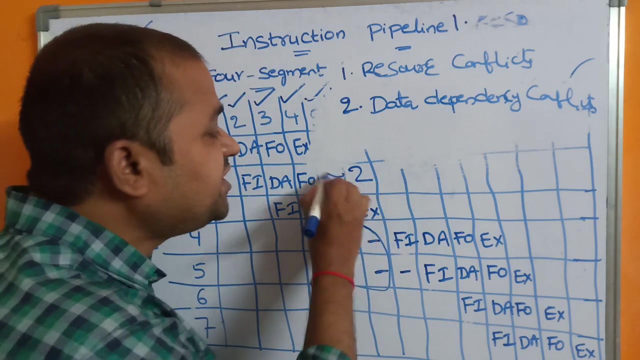 So data dependency conflict means when an instruction depends upon another instruction but that instruction is not calculated till now. So let us have a second instruction, But the second instruction depends upon the 1st instruction, upon the first instruction, but this first instruction output is not calculated till now. 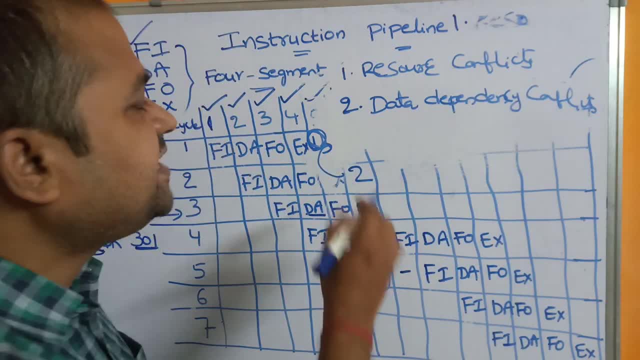 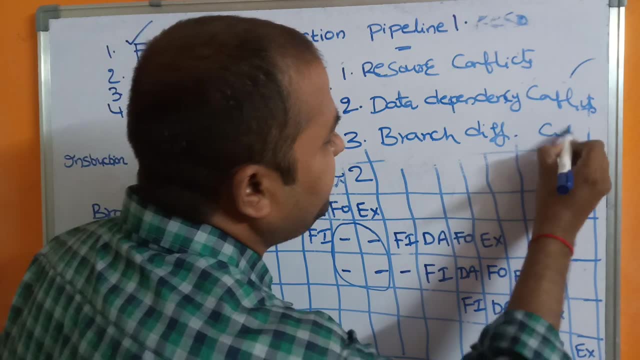 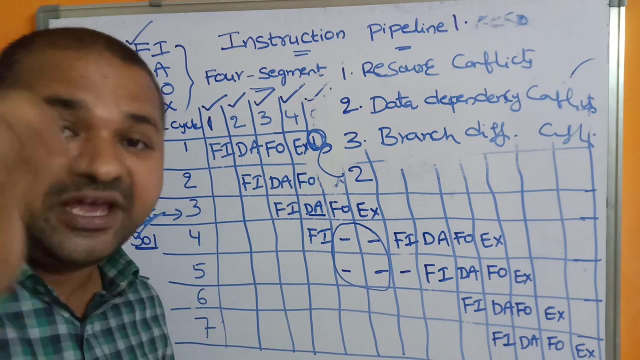 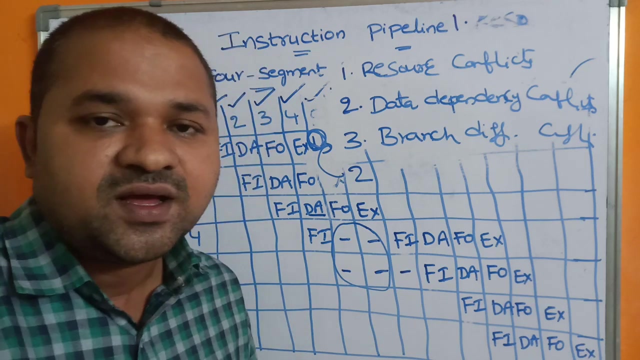 so that problem is called as data dependency conflict. and the third problem is branch difficulties conflicts, branch difficulty conflict. so already we have seen that example here. so whenever we are executing the branch instruction, if the condition is satisfied, then the program counter will be loaded with a new address, a new branch address, whereas if the condition